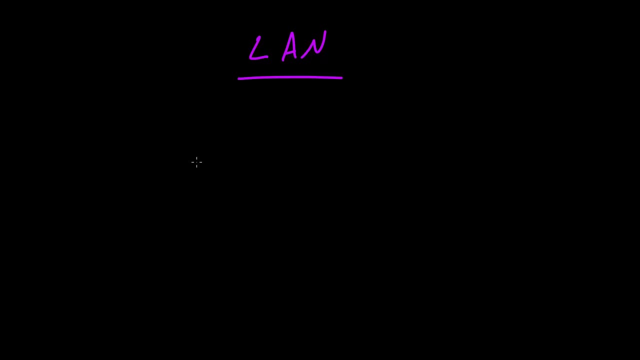 local area network. Well, what type of computer network does this represent? Well, a local area network pretty much means that all computers are in the same building. So here's your building. right now You might have a computer here here. alright, computer, computer, computer. 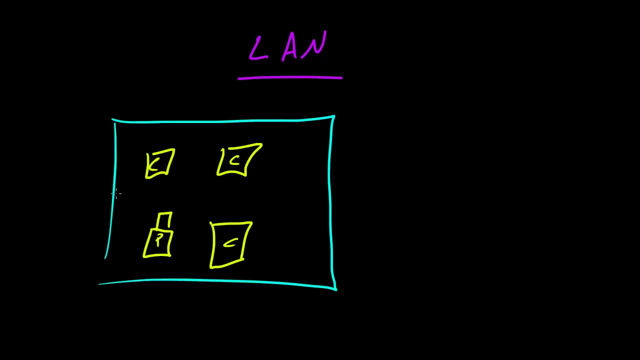 and you can, you know, of course, have a printer. That's a type of computer too, as we talk about. So you might have a computer here, here, alright, computer, computer, computer, and you can, you know, of course, have a printer too, as we talked about earlier. But basically LAN. 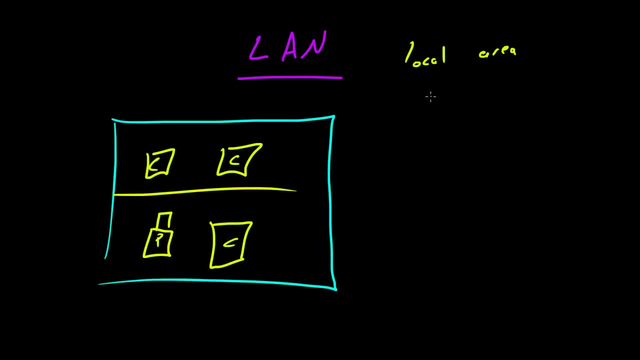 which is a local area network. This is how you know if your network is a LAN. All the computers are in close distance to each other and they're usually in the same house or same building. Again, the building could be either a house or a high school, or even you know. 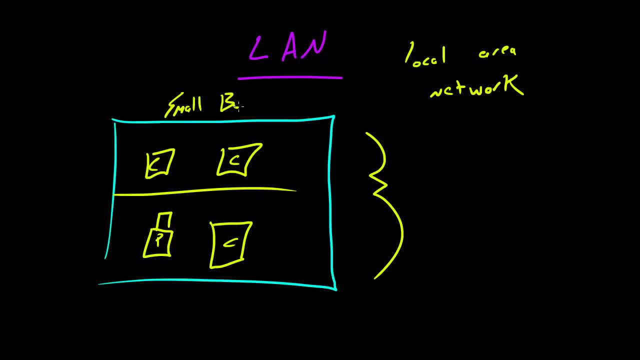 a small business, So say that this is a small business, right here. This would be an example, example of a LAN. Now, why would you want a LAN? Why would you want to connect the computers in a high school or, you know, even in your home? Well, it's good to say this was a college. It would be. 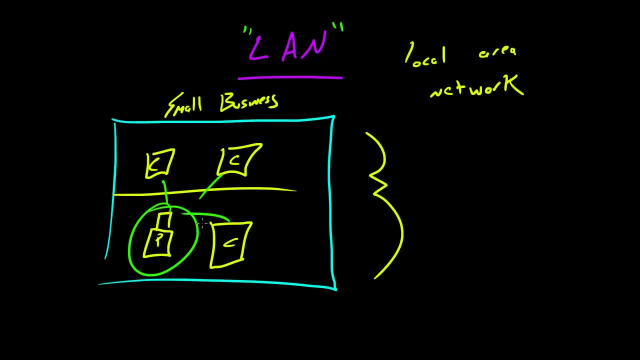 really good for sharing printers And that's how colleges whenever they connect them in this type of network. that's why every you know computer in your computer lab it doesn't need its own printer. So that's one you know very useful technique of a LAN. Another thing is you know 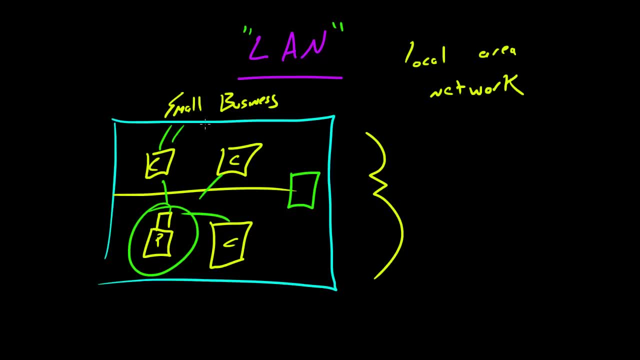 if this was your house and you know, maybe your mom and dad had a computer, maybe your sister had a computer and you had a laptop- what you could do is you could actually hook this up to the same server. Oh, Dan, be quiet, I'm trying to teach here And basically all of you guys can store. 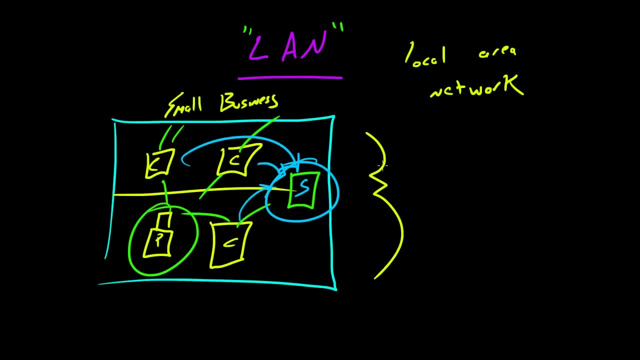 your illegal movies on that same one server, So that's really handy. But anyways, good for sharing things in small or the same building in a close-up, And these are usually connected by cable or wireless. Okay, I got to let my dog out, Sorry, guys.